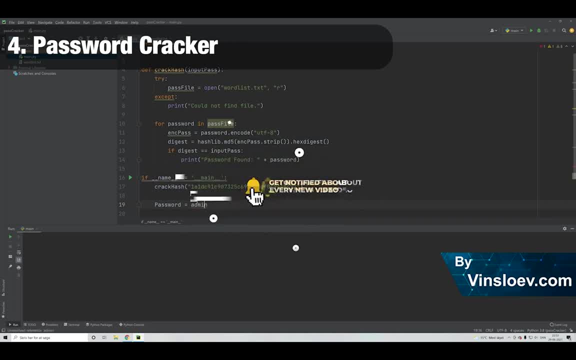 tracking. Well, we will crack hash password, which is also known as a dictionary attack. So this is the common attack approach that hackers use. when they have gotten access to a database of passwords. They are hashed, but we will learn how we can de-hash them by having a dictionary of known passwords. 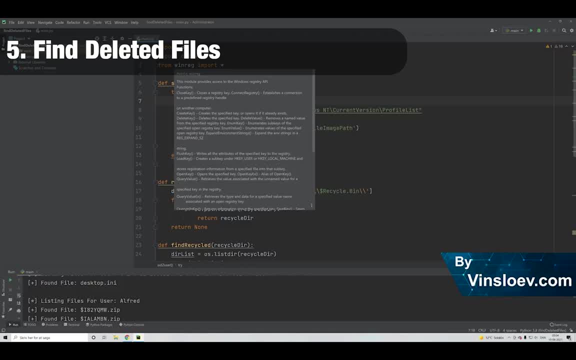 Number five. So this Python project is about finding deleted files. So we'll build a script that can be used to find deleted files on a given operation system and sort them based on the user who deleted the files. So if you have gotten access to a computer or you just want to find some files that you might have deleted yourself, 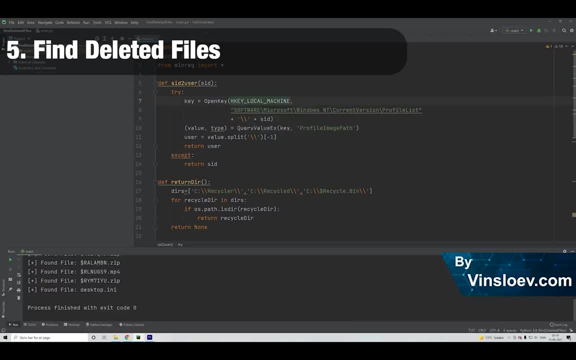 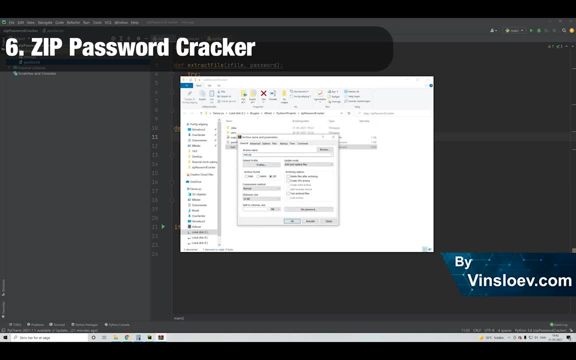 you can use the script to recover the files if somebody has tried to hidden something on the computer. Number six: ZIP password cracker. So this script will enable us to crack ZIP files. that is password protected. So we will have a list of passwords. 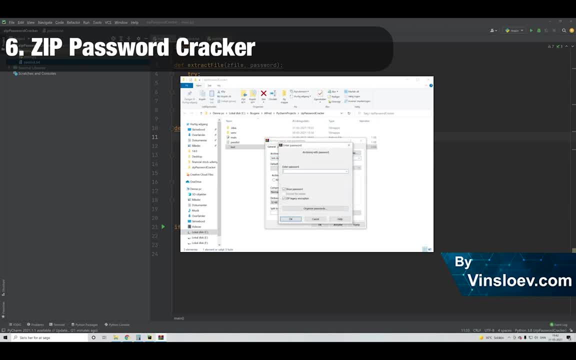 which is also referred to as a dictionary tag, similar to the project number four, But here we'll use that dictionary tag approach to try to crack a ZIP file that we have received that is password protected. So we'll create in this file or this video, 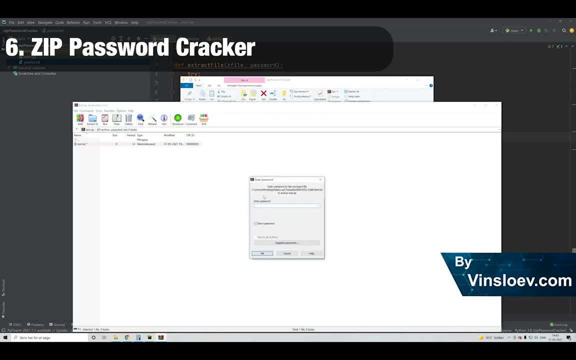 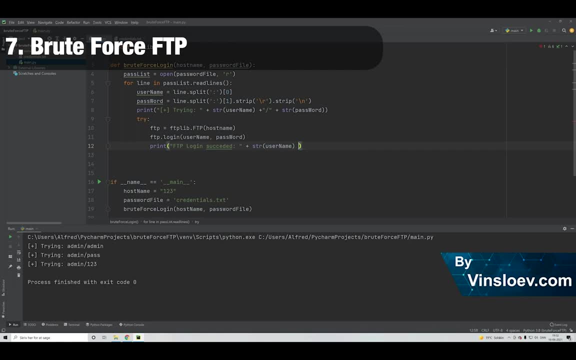 a ZIP that is protected, and then we'll just try to break it using our list of passwords, Number seven. Here we'll try to brute force our way into FTP. So instead of trying to use the anonymous login, which we saw on a previous project, we'll this time 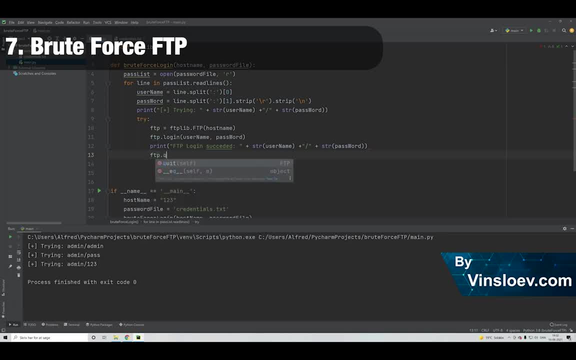 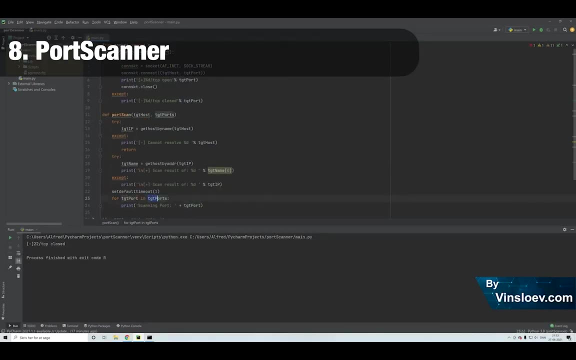 have a list of known usernames and passwords and simply just brute force our way by trying all kind of combinations of these until we hopefully hit the right combination of user and password. Number eight Port scanner. So this script will allow us to scan a given server for open ports where a connection can be made. 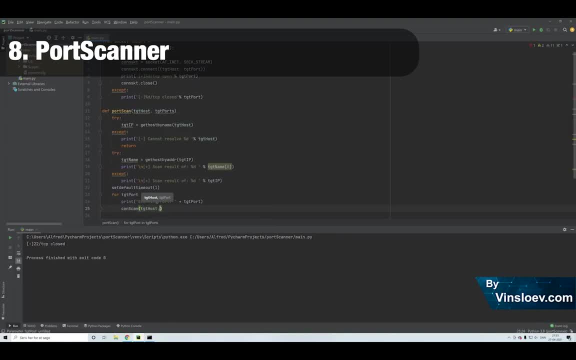 Usually you want to have all the ports that you don't use closed, but in most cases people might leave a port open that allows an attacker to go through that port. So this can be used on your own server or to scan a target server.